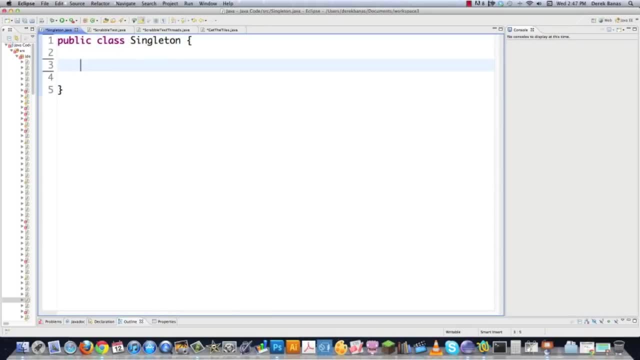 it, singleton. Now you absolutely don't have to do that, but in this situation it makes sense. Like I said before, singleton pattern is just going to force you to only have one instance of a class created and then this guy, private, static singleton, first instance is going to hold the one and only instance for the 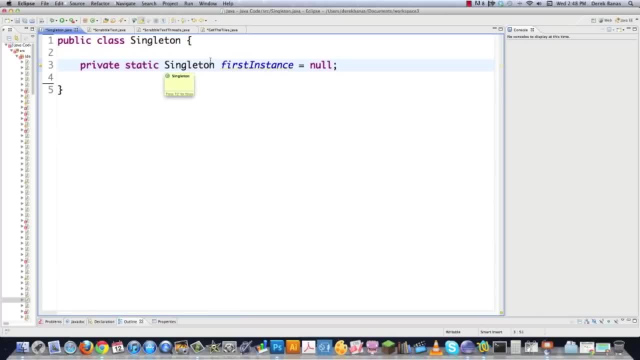 class singleton. So this guy is going to be the access point for any object or the one object that's going to be created from this class, and it is static in this situation because objects like this will almost always need to be available on a global basis, So that's the reason why that is set as 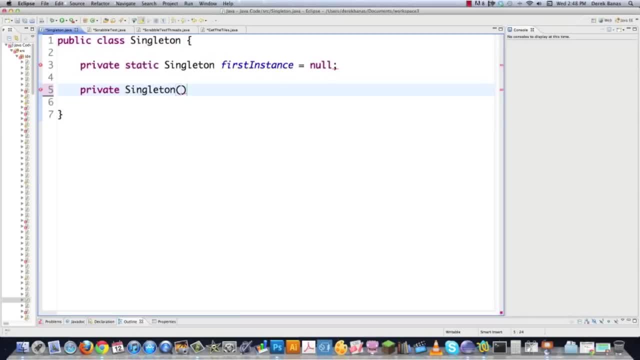 static, And then we're going to come in here and go private singleton and make the constructor class private. And the reason why we're doing that once again is to make sure that there is only one instance for the class singleton. And that is the reason why we're going to have that be private, because if they try to 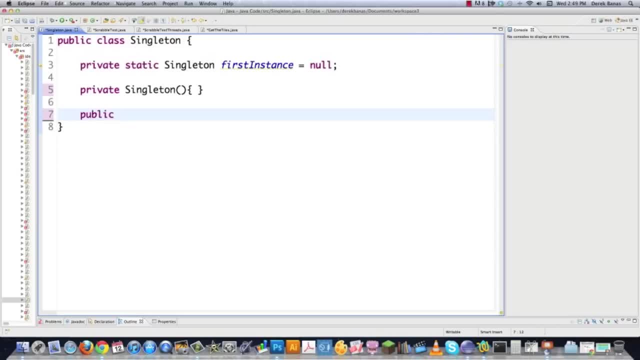 create a new one. it's just going to create an error, And then what we're going to do is go public static singleton, get instance and get instances almost universally used as a method for the singleton pattern, And basically what we're going to do inside of this guy is: 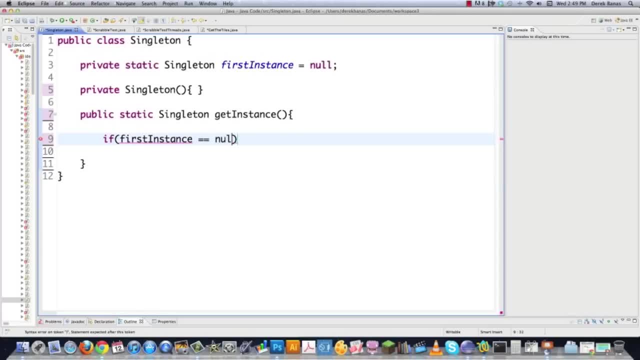 check if first instance is equal to null, or whether it exists or not, which means it wouldn't be null if an object was created for it. So we're checking in that situation And if so, we're going to go. first instance is equal to new. 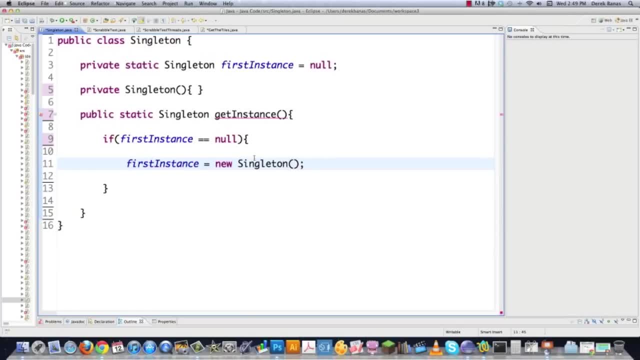 singleton right like that. So the only way they're going to be able to come in here and create a new singleton object is if one doesn't exist already and that one would be stored in this field up here. And this right here is known as lazy instantiation, And what that basically means is if the instance isn't needed, it is never going to be. 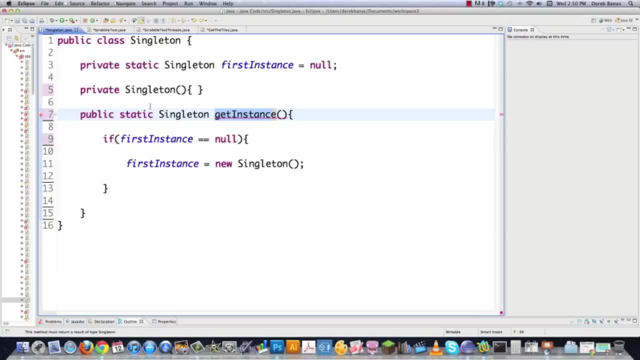 created. So the other way it's getting created is if get instance is called And then, after we're done with this, we're going to go return first instance. So you can see right there that something's going to be returned every time if first. 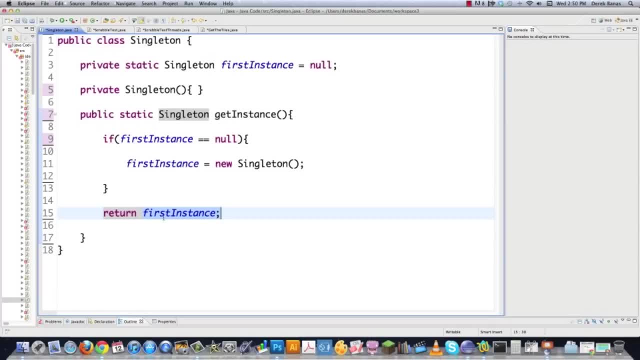 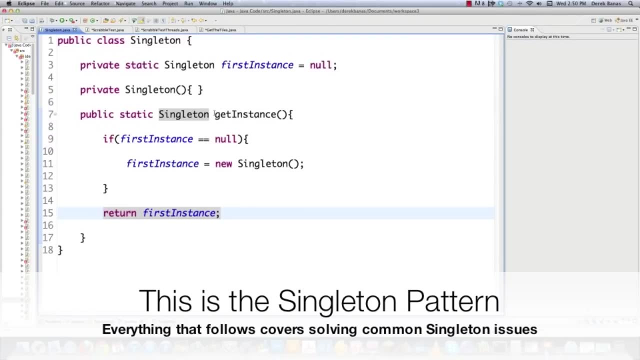 instance already exists and they try to create a new singleton object, it's going to return the one that is already created. Otherwise it is going to create a new one. So there it is: There's a singleton pattern. However, we're not done, because there is one thing that is always covered with the singleton pattern, and that is: 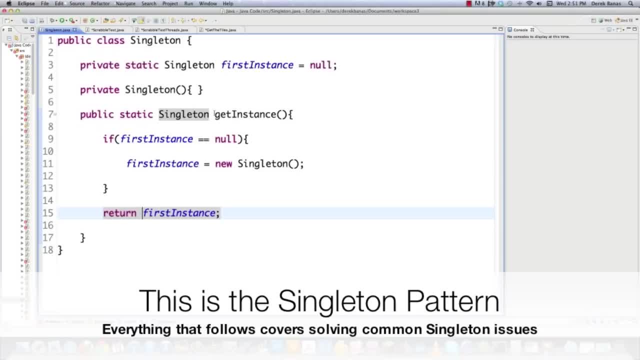 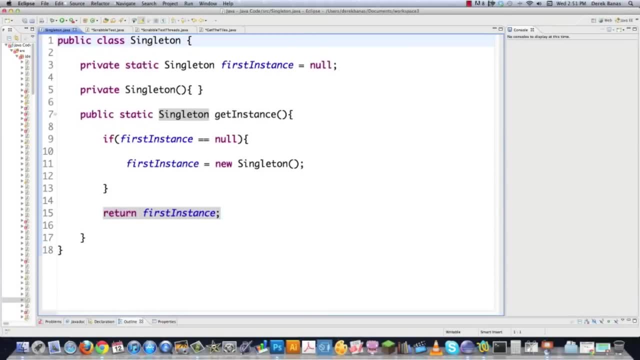 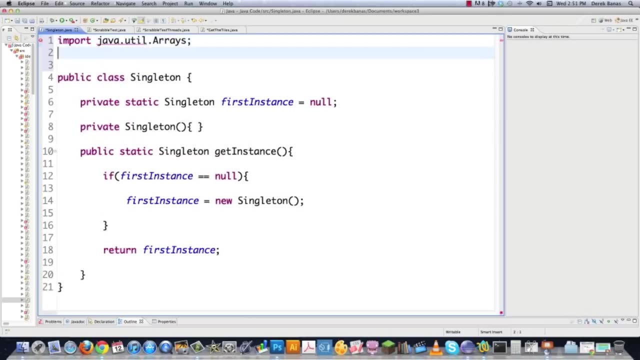 basically, what are we going to do in a situation where we are dealing with threads which could potentially create more than one object, whether we try to block that or not? So this guy, I have to implement my little Scrabble thing that I talked about before. I'm going to go import Java utility and I'm going to need the arrays library and the collections which I'm 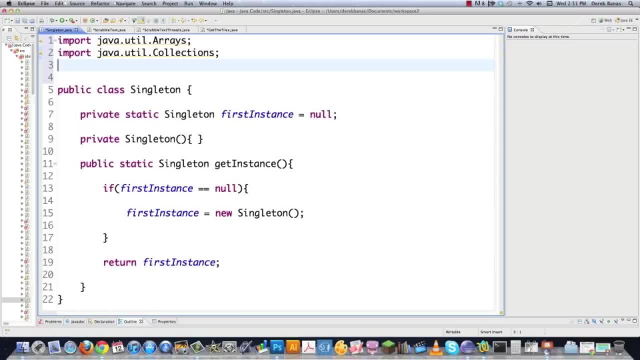 going to use to jumble up all the letters that are going to be stored in inside of a linked list. So that means I'm going to need linked list. I'm actually doing this also because I've received a bunch of questions in regards to arrays, collections and linked lists, So I try to cram multiple tutorials into one. So what am I? 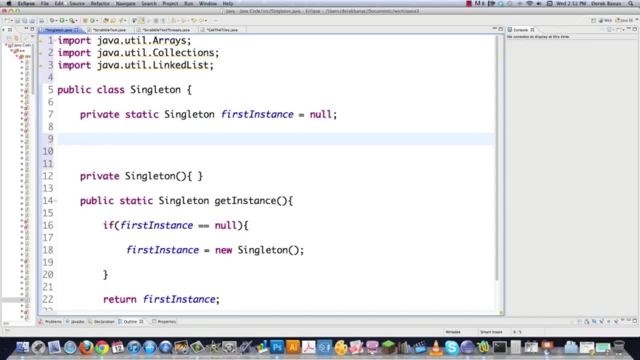 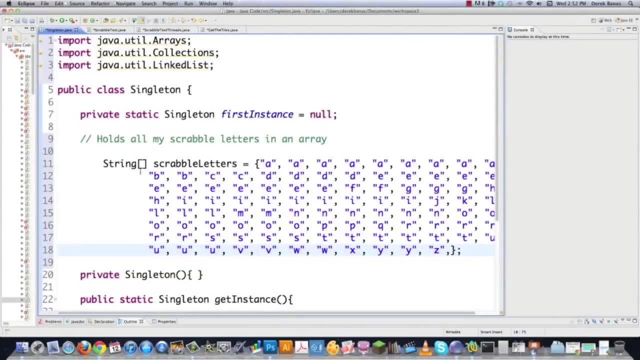 going to need to do here. Well, after this guy right here, I'm going to need to come in here and actually get all of my potential Scrabble letters. Well, I have that saved elsewhere, so I'm going to grab that. And here they are, and I pasted them in there. 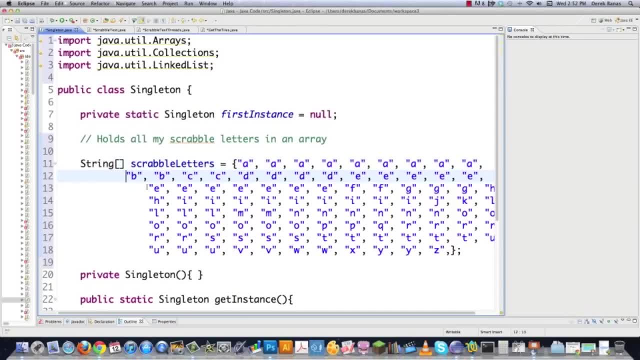 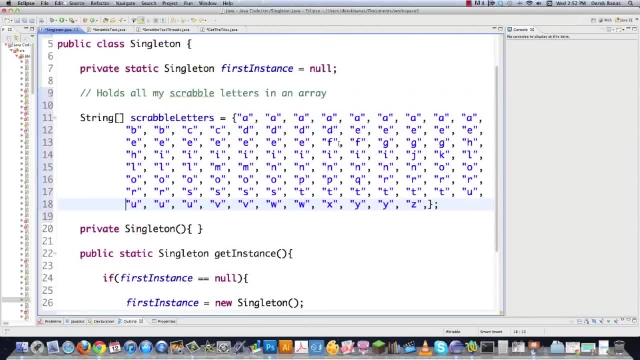 And that is all they are. Those are all the potential letters you can have inside of the game of Scrabble And I didn't see any reason to type those out, but I'm going to clean them up a little bit. So there you are. That's what we got right there. 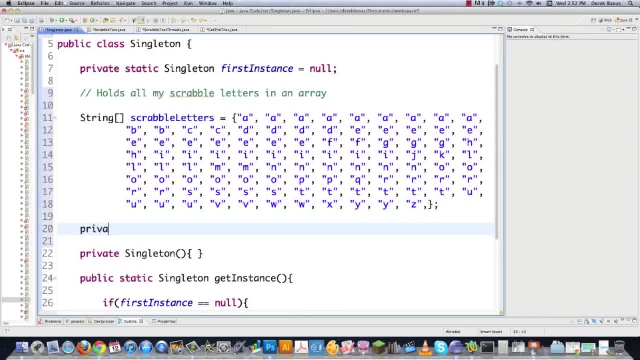 Just a whole bunch of letters. Then after that I'm going to go private linked list and I'm going to store all these letters as strings and I'm going to call them letter list And this is going to be equal to new linked list, again string, And then I'm going to take all of the letters in. 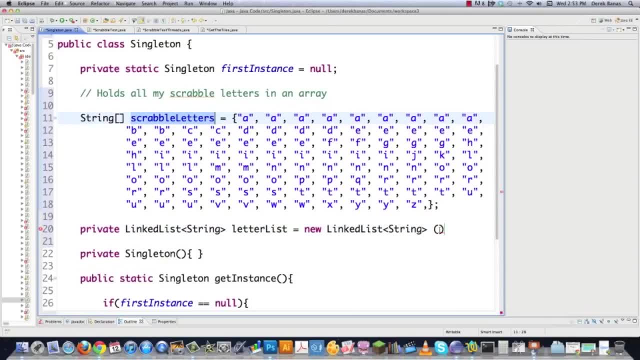 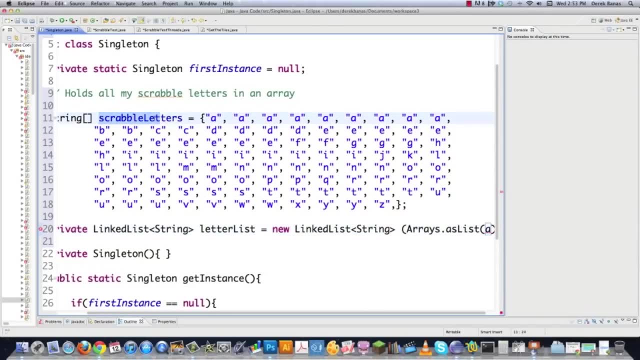 this array that we have right here and I'm going to throw them into the linked list. So we're going to go arrays. If you wondered how to do that, you just go as list And inside of that you're going to type in Scrabble letters. So that is a question that I recently received: How to get a array of things. 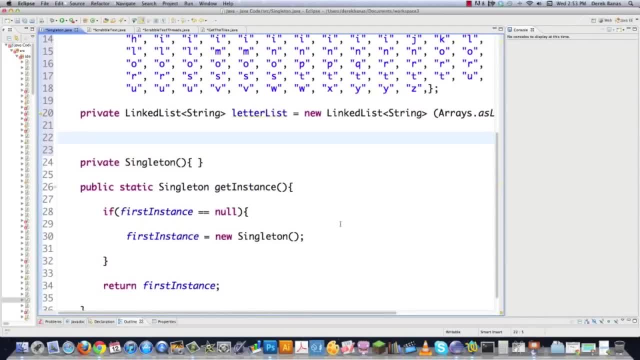 inside of a linked list. And now you know, And all the code is available underneath this video. if you want to go get it, Then what I'm doing- because I'm going to be working with threads- is I'm going to create a static boolean And the first thread that is going to be created is going to be: 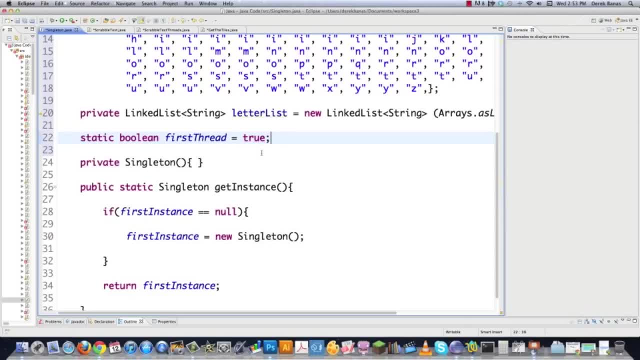 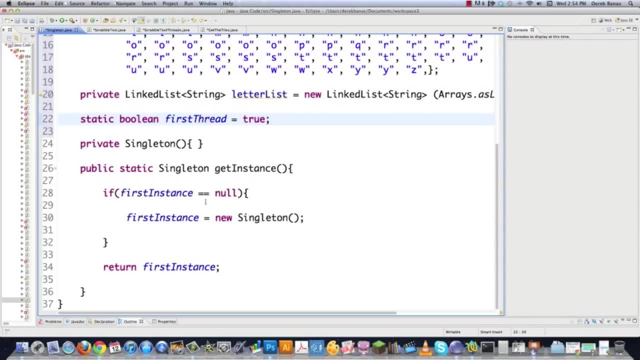 slowed down so that there is the potential for a second thread to come in and cause masses of disaster- And that is exactly what that line is going to do There for me- Then we need to come down inside of this guy and start creating some disaster. I'm going to say, if first thread, which is going to be 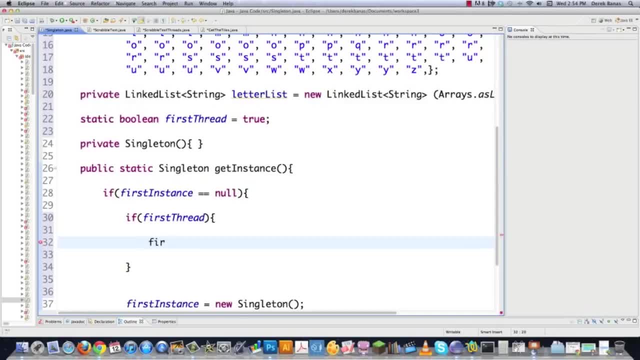 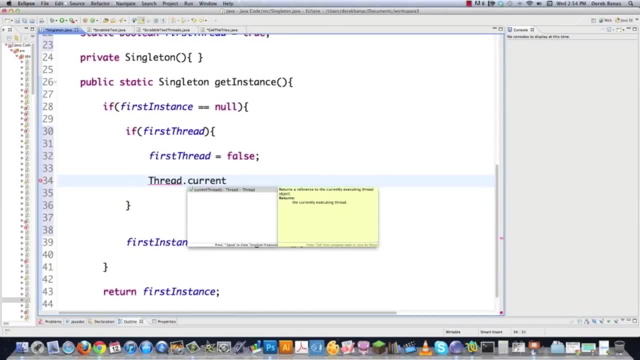 true, Then I want to perform some things that are going to slow down my thread. So I'm going to say, first thread is equal to false, I'm going to change it back to false, And then I'm going to go thread current thread and I'm going to cause it to sleep, And what this is basically going to do for me. 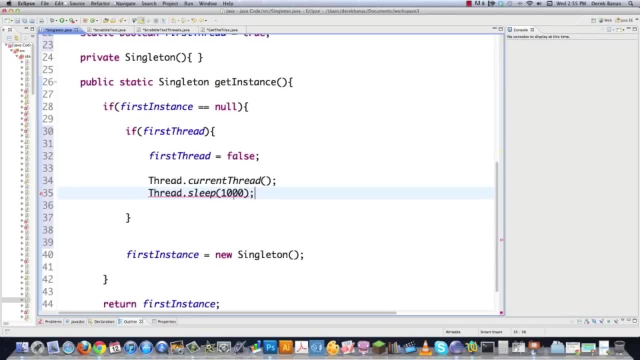 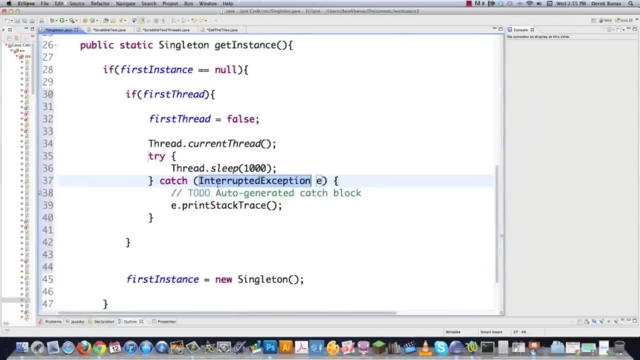 is going to give the other thread that I'm going to be creating the opportunity to cause mass disaster And if you scroll in here you'll say it needs a try catch block. so I'm going to say: surround with try catch block to save myself some time. Everything else here can be. 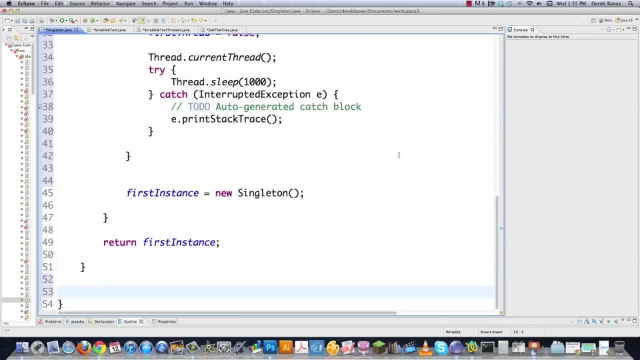 exactly the same. However, I'm going to come in and create a whole bunch of other different methods inside of here that are going to work with these threads to create our little Scrabble game that we are going to be creating here. I'm going to go public and what this method is going to do is: 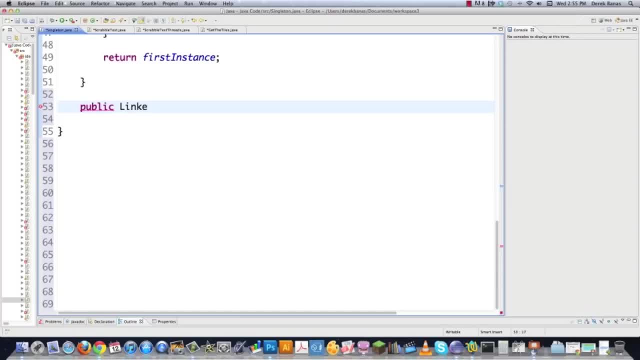 return a list of all the available letters. So I have all those letters in a linked list and they are all strings. So I'm going to call this guy get letter list And what's it going to do it? This is how you would return fields inside of a singleton. You're just going to reference. 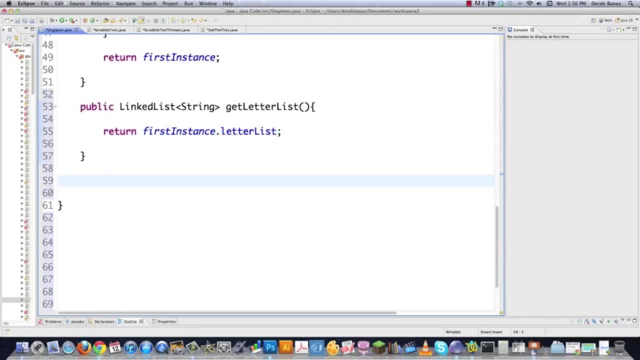 letter list in that situation. Nice and simple. So let's create a couple more methods here. I'm going to create this guy and it's going to get tiles for my player. So it's going to return a string linked list and it's going to be called get tiles and it's going to receive an integer. 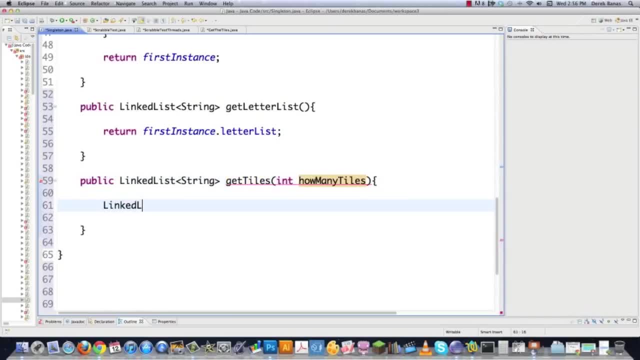 It's going to say: how many tiles do you want, and then I'm going to create another linked list. It's tiles to send and be equal to new linked list. If you want to really really understand this, you definitely should get the code Almost every single time I get an error from one of you. 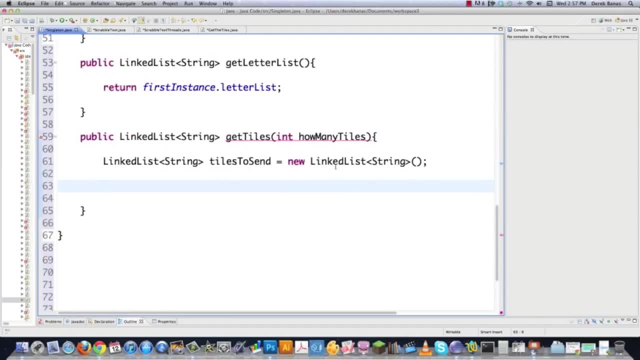 guys, or not understanding why something is done a certain way. it is because the answer is in the code, but you didn't see it. And then we're going to cycle through the linked list, while adding the starting strings to the list that's going to be returned to the user, and then, at the same time, 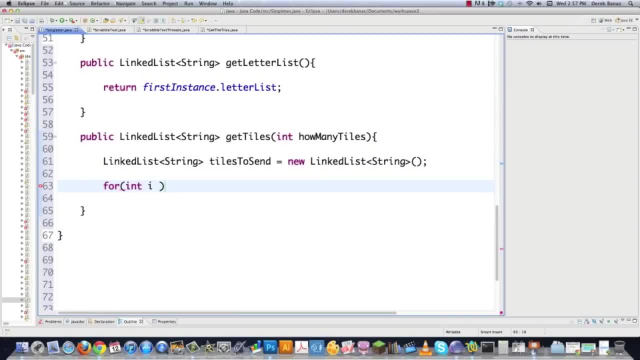 we're going to delete them from the beginning of the list. So to do that, you're going to int. i is equal to zero. We're going to start at the zero index and we're going to go while i is less than or equal to how many tiles they requested, and then we're going to increment. So no big deal. 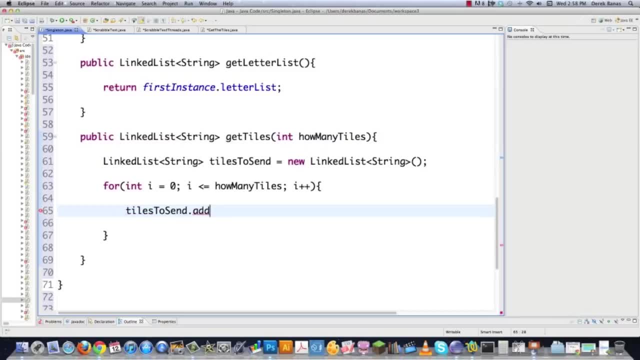 We go tiles to send, So tiles to send is going to be going back to the user. So if they say, hey, I want seven tiles to start this gravel game, it's going to kick back seven letters and then chop those seven letters off of the linked list so that nobody else gets them. How do we get those guys? 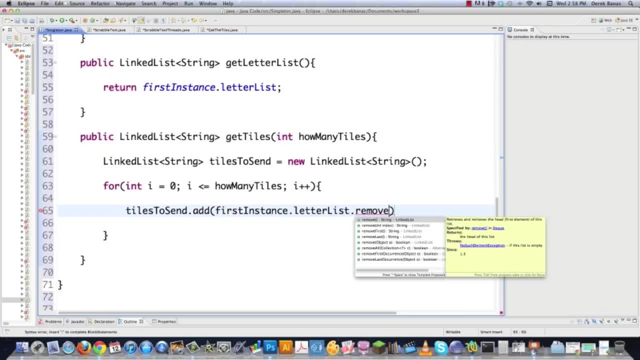 We're going to go first instance letter list and we're going to remove- and you would have thought I'd put an i in there, but I know I'm going to put a zero. and the reason why is, whenever you call remove, it is going to chop off the zero index and then move everything from the right over to the 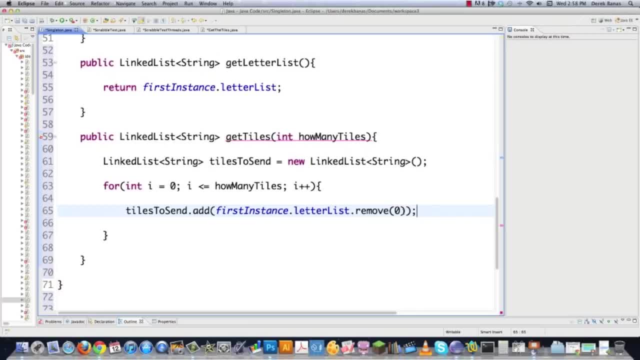 left. So next time through, what is in the one index will now be in the zero again and everything's just going to work out perfect. And then, after it goes through all this, it's going to go return tiles to send and that new array is going to be sent back to the function that called it All. 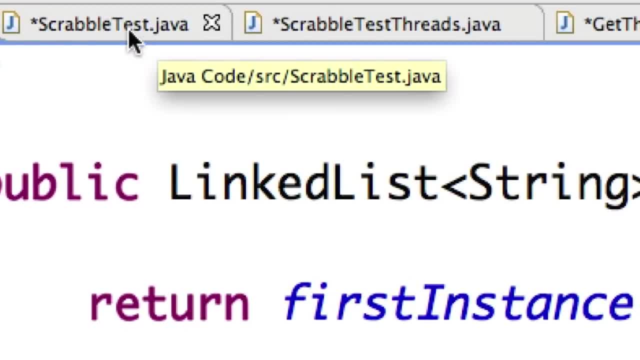 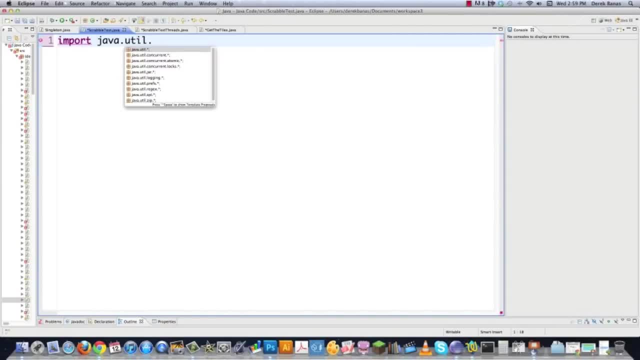 right. so everything's set up there. So now we're going to go into Scrabble, test java Right, like that, and we're going to start playing around with this guy. So what are we going to need? We're going to need import java utility. We're going to need linked list because we're going to 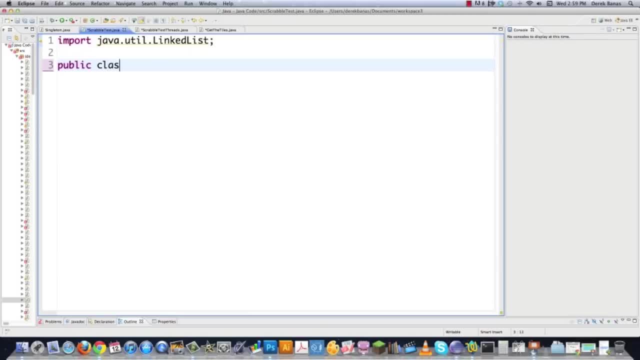 be playing with linked lists again inside of this guy I'm going to go public class Scrabble test. public static void main string, because we're going to be executing everything from inside of here Anytime. you see main from now on in my tutorials that would. that's exactly what it means, So we're. 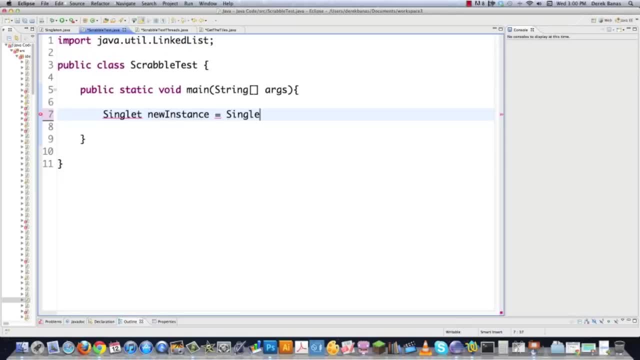 going to go to singleton, new instance is going to be equal to singleton and we're going to go get instance. This is part of the singleton pattern and that is how you're going to create new instances of the singleton class, Right like that. Let's say, we want to print out a unique ID for all of our instances. 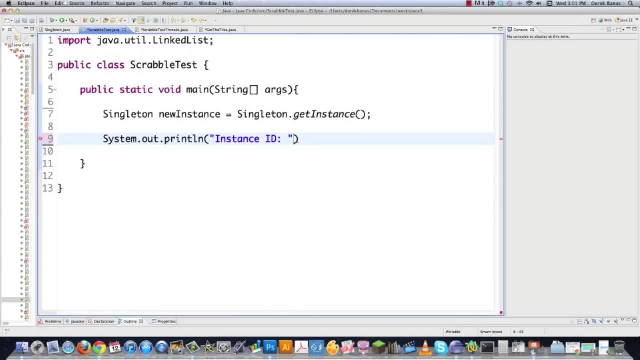 that are going to be created. I'm just going to go instance ID and, if you want a unique ID, just going to go system identity hash code. And what are we going to put inside of here? New instance, which is the name of this guy's, going to be created for us And that way we'll be able to track. 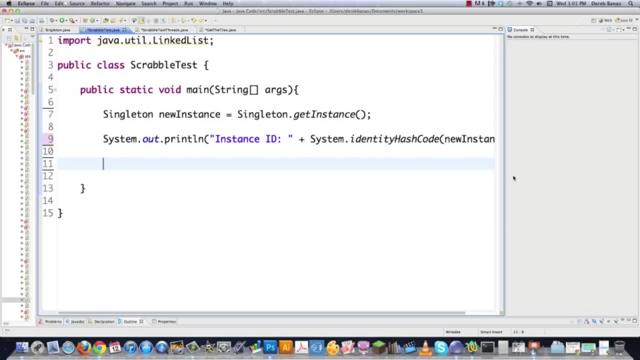 whether we are dealing with the same instance or not. So we're going to go create new instance: Same objects, or whether we're dealing with different objects, which is important, And this also helps you with debugging and a whole bunch of other different things. So then, what are we going to do? 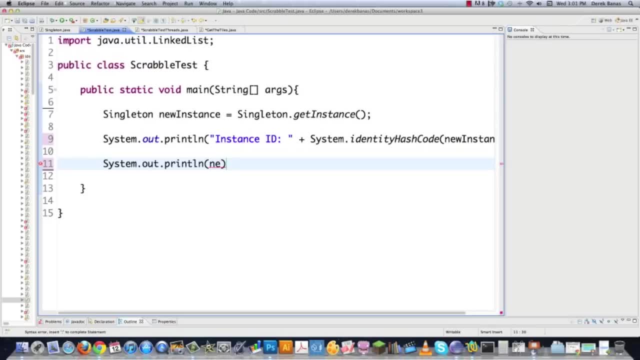 We're going to get all the letters that are stored in the list and we're going to print those out on the screen. So how do you do that New instance, get letter list, which is a method that I just created here a couple seconds ago? Flip back, if you don't remember it? Of course, this is new instance And 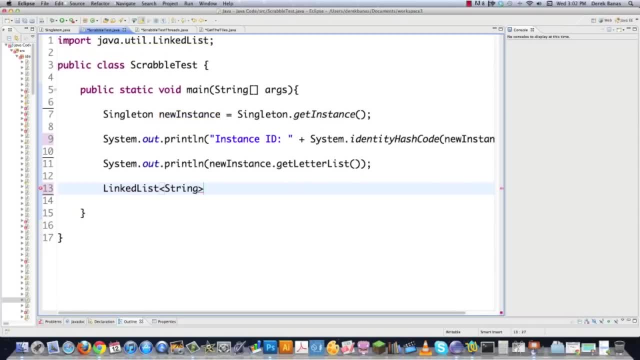 then I'm going to go linked list and this is going to be a string just like before, or a group of strings, And I'm going to say player one tiles is equal to New instance get tiles and I'm going to say I want seven. We're going to act like this is the 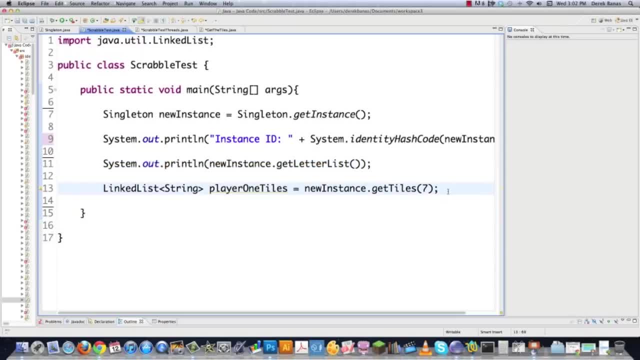 beginning of our game And then let's say we want to print out to screen all the new tiles that player one just received. That's useful. So we're going to go player one and then player one tiles and that's going to print out all the tiles for player one in our Scrabble game. And maybe we also 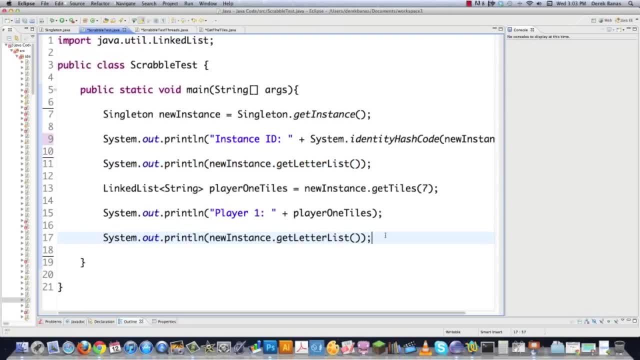 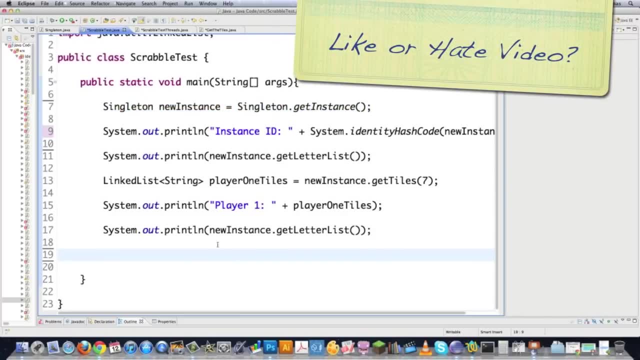 want to print out our letter list just to see how it's changed since player one went in there and created that guy, And then what we're going to do is go singleton again. We're going to try to create a new instance. This is going to be our second player and I'm going to call it instance two in this. 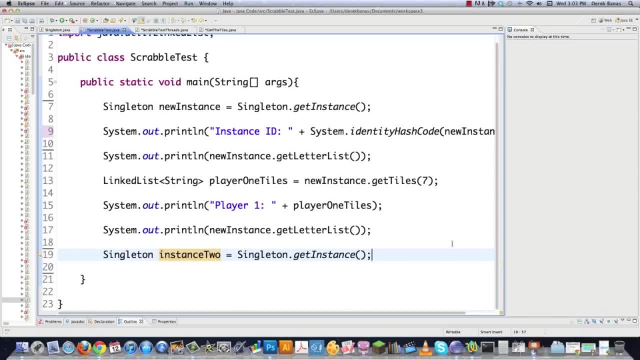 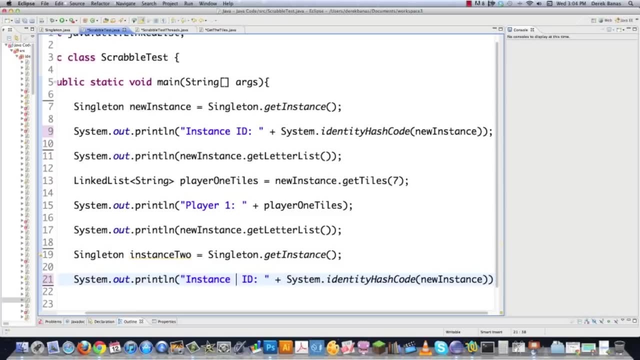 situation. We're going to call get instance just to see exactly what happens. And then let's say that we want to also come in here print out a unique ID for this new guy. Let's call this instance two ID. Let's call this instance one ID. So we're going to see if those values changed just because we 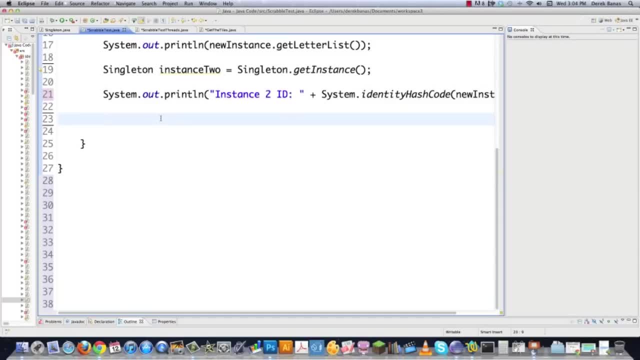 created a new object, even though they're not supposed to. Of course, I think you probably know the answer. We're also going to show you how to break it. And then let's go and print out our letter list again just to see how things have changed. And then I'm also going to 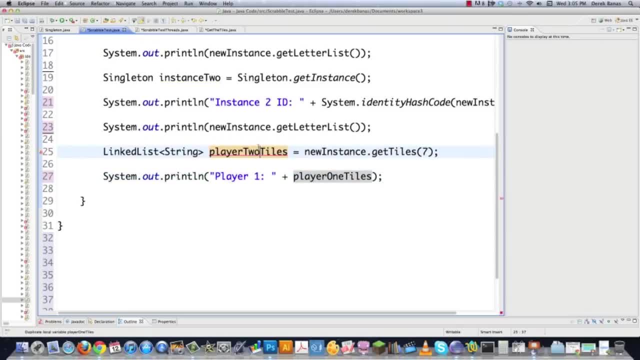 copy this and print this out. There's that Call this player two tiles. So player two is going to get a new set of tiles, which is going to work, by the way. And then there are player two's tiles And if we file save this, we're actually going to be able to execute it. You're going to be able to. 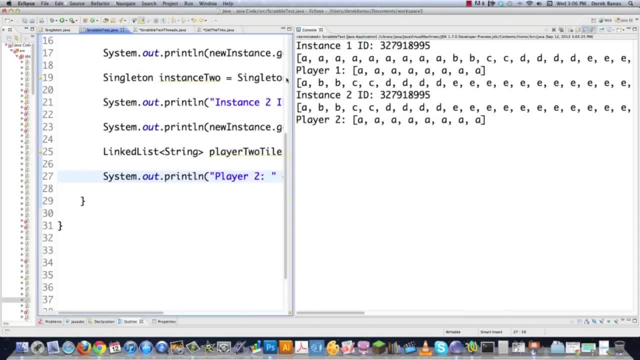 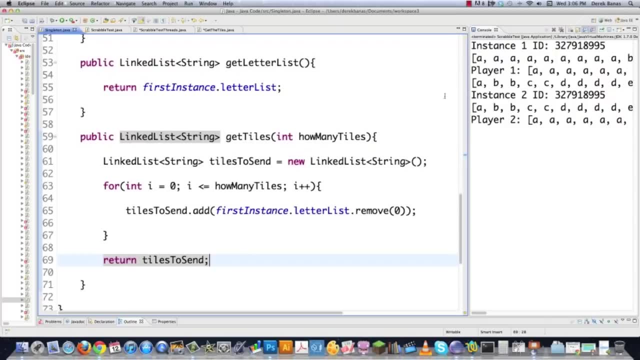 see some things here And there are all the letters printed out, but that's kind of messy. What I want to show you here is, instead of that, I'm going to go over into singleton, I'm going to scramble these letters out so that they're not printed out, all in order, because I think that's a. 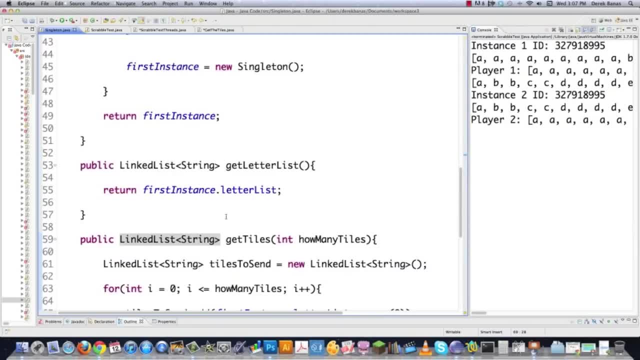 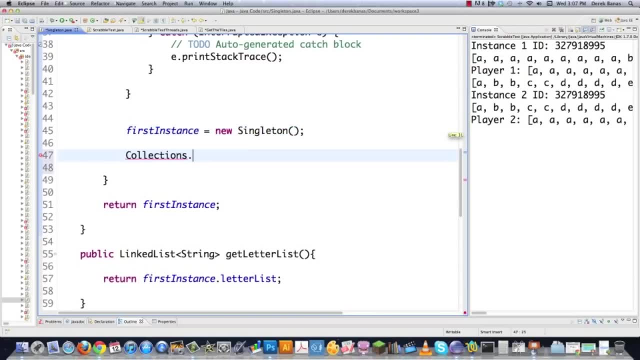 little bit more impressive. So I'm going to jump back into singletonjava and right here, where we get to first instance, where we created our first object I'm going to call collections and I'm going to shuffle first instance, which is this guy right here, so that all the letters are not in order. 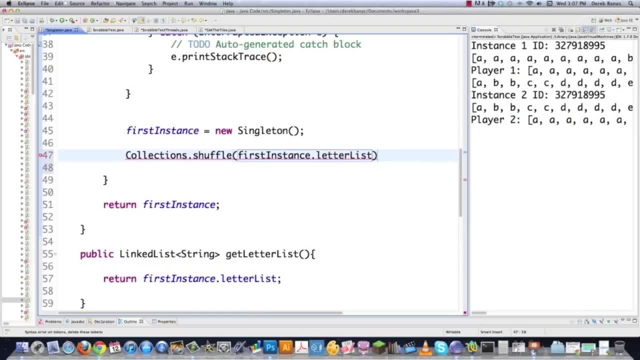 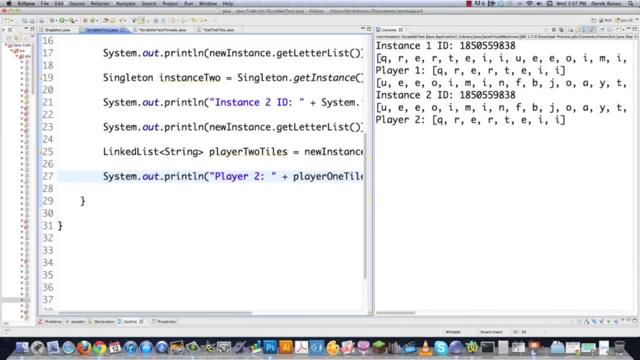 that they're going to be all randomized- See QR, And then you can also see the user getting the right letters. So if they want seven, that's one, two, three, four, five, six, seven, Right like that, And you can see that they got those same seven letters right here And then everything is moved. 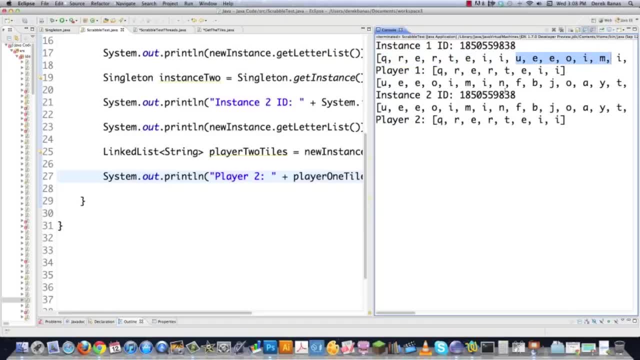 over thereafter And then you get all this other stuff going right there And you can also see that the instances for these two objects, even though two separate objects were trying to be created, you can see that the same object that represents the letter list is identical. So there's that. So 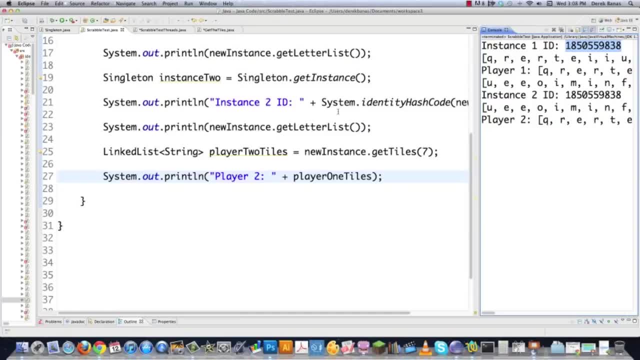 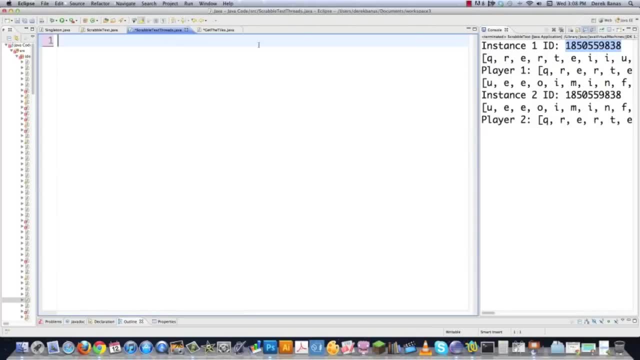 what happens if we come in here and we start implementing these different players as threads. Now you're going to see, I'm going to create a new class called Scrabble test threads right here And I'm going to implement that. So I'm going to go public class Scrabble test threads And we're 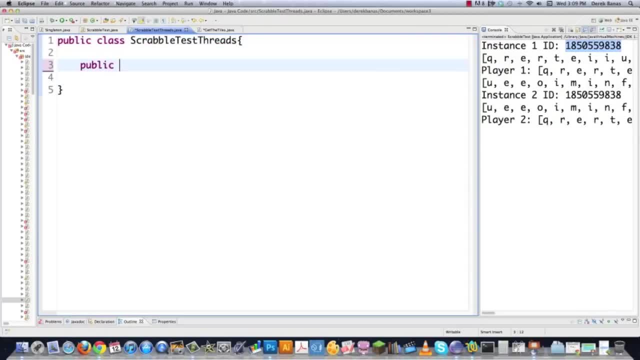 going to get another review of threads, because I get asked about them all the time- And public static. What is this telling you? This is telling you that this is going to be a main execution area. Why? Because I'm using public static void main, So the first thing I'm going to do is go in here. 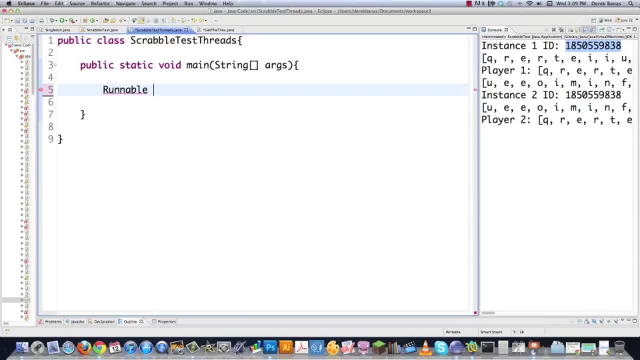 and go runnable and create a new thread using the runnable interface And this is going to execute my code. for me meaning the code for creating new instances of the singleton class new and get the tiles is going to be the name of the class that's going to have the run method inside of it to use. 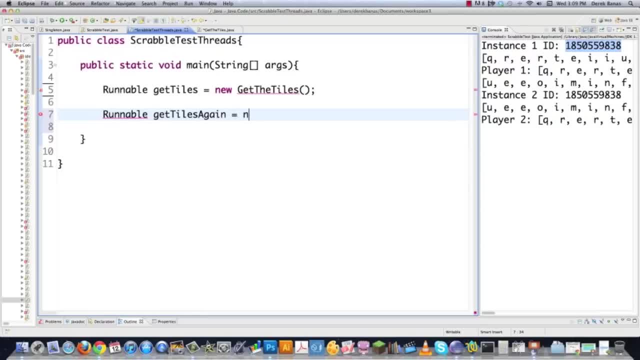 with this thread. get tiles again is going to be another thread, and get the tiles is going to be used again, which I'm going to create here in half a second, And then I just need to call for the code inside Of get the tiles to execute, And it's pretty simple. I'm just going to go get tiles and call. 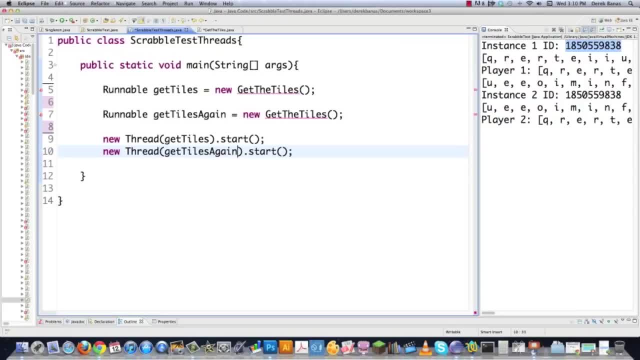 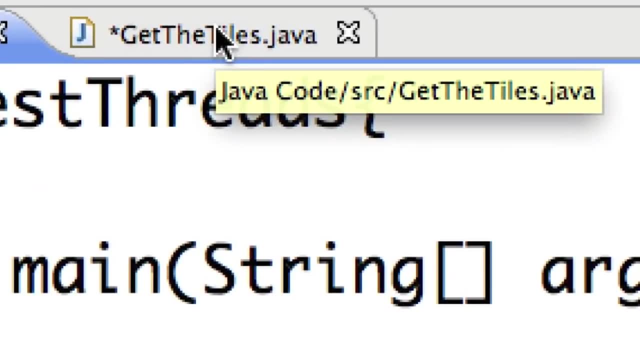 start on it. And there's that, And then this is going to be: get tiles again and start And that is it. So if I'll save that and that is going to execute all of my threads. So now we need to go into get the tiles, dot Java and start playing around with threads and see how threads can very 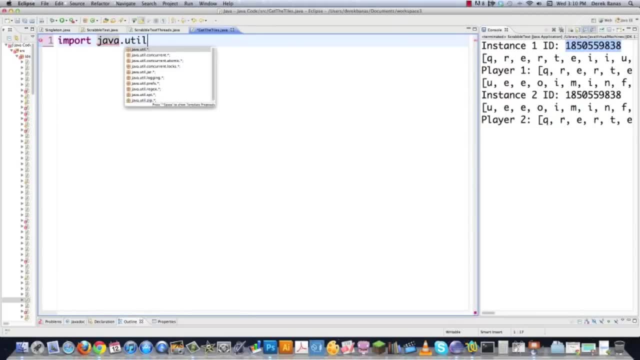 easily and quickly start destroying things in regards to using the singleton pattern, And I'm also going to show you exactly how to block them from doing so. So when we create a new linked list or grab information from the linked list library- and I'm going to go public class- get the tiles. 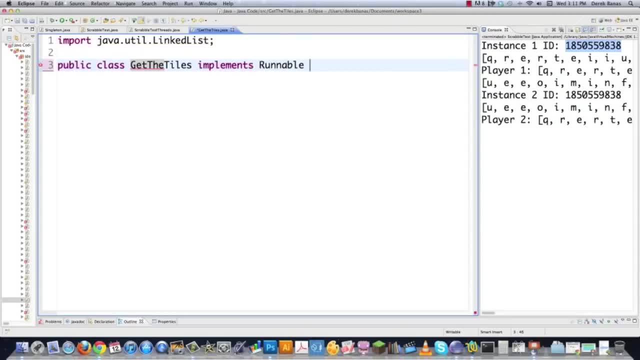 implements runnable because we're using those threads And then we need to go public void run And then we're going to go singleton And these. this run method is going to execute all the code in here for both of my threads, if you forgot previously. So I'm going to go create a singleton. 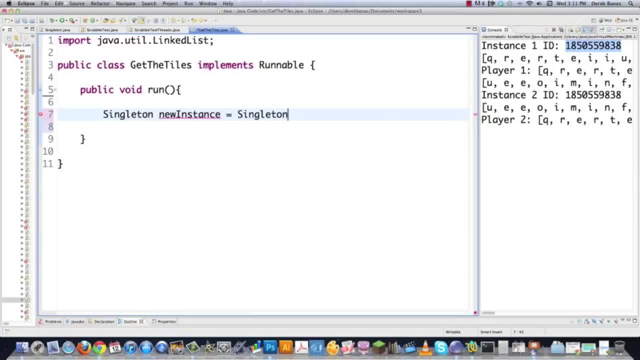 object called new instance and it's just going to be singleton, get instance Again. that's how we're going to create all our singleton objects And then we're going to go linked list string And this is going to be a player. I'm going to have this be player one. 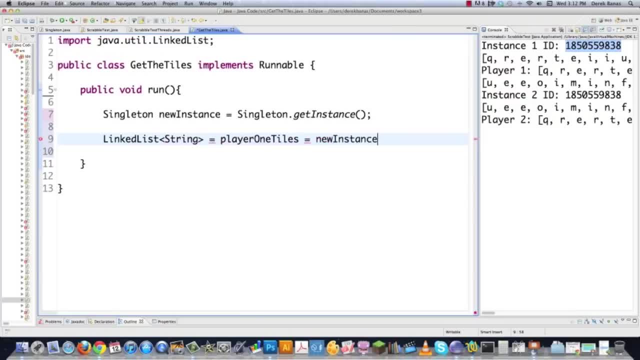 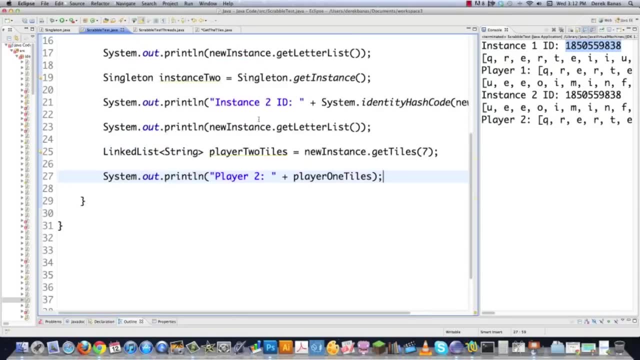 tiles, even though there's going to be two players, is equal to new instance get tiles And we're going to get seven tiles, just like we did previously. And actually I'm going to steal from Scrabble test some code so I don't have to type it out. I'm going to come in here and get. 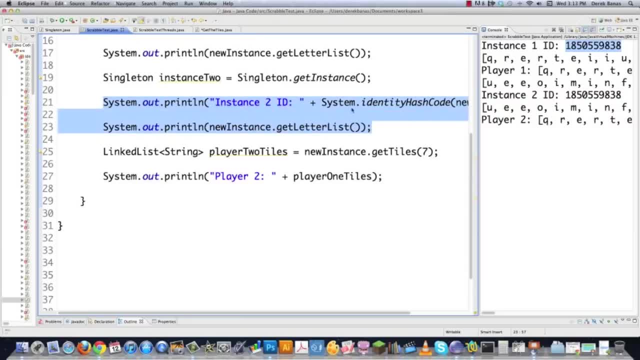 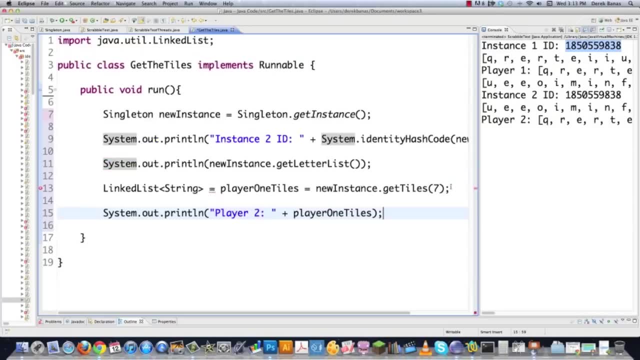 this unique ID And I'm also going to get the letter list. So let's copy that bounce inside of there and then bounce over and Scrabble test again and also copy this guy right here and paste that in there. And I'm just going to go instance ID and take player and put that inside there And then 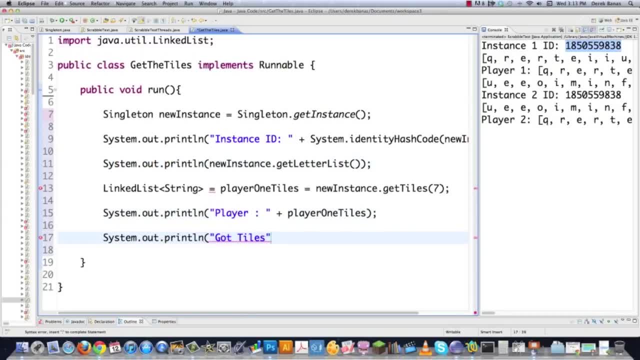 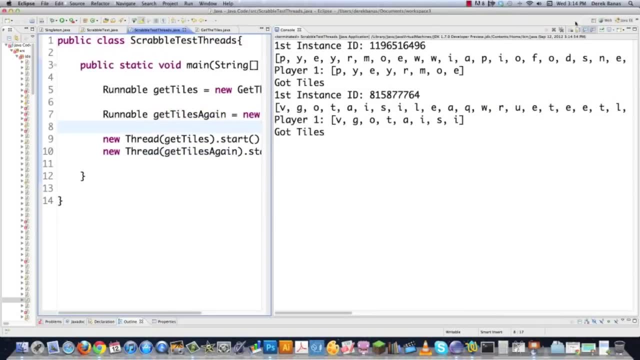 let's put another message inside here. Got tiles? There we are And we can file save that. And now we can test this guy using threads. So let's file, save it and it's executed And there you can see using threads. What we got here is our first instance of the object. Look at that. The ID is: 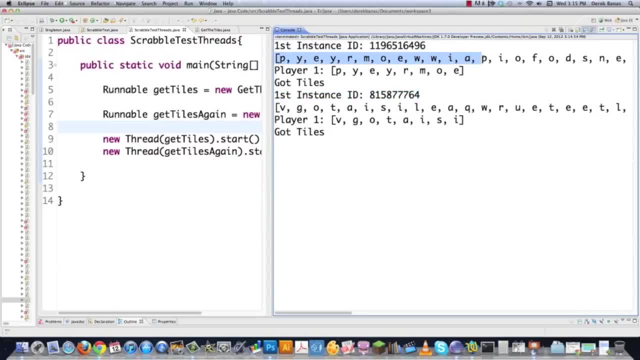 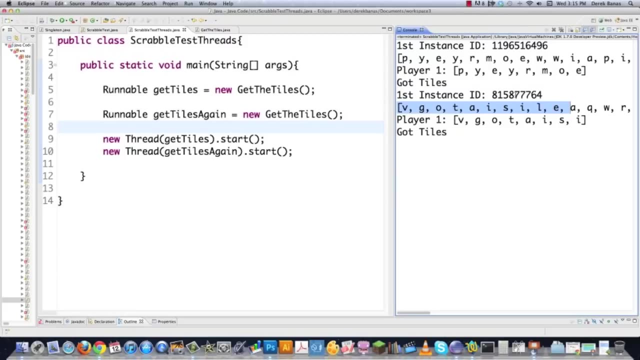 instance object that was created And you can also see that the list of letters are also completely different. So even though we tried to prevent it from being able to go in there and create multiple different threads and multiple different instances of different letters, which would obviously completely destroy our Scrabble game, it did go in there and mess that up either. 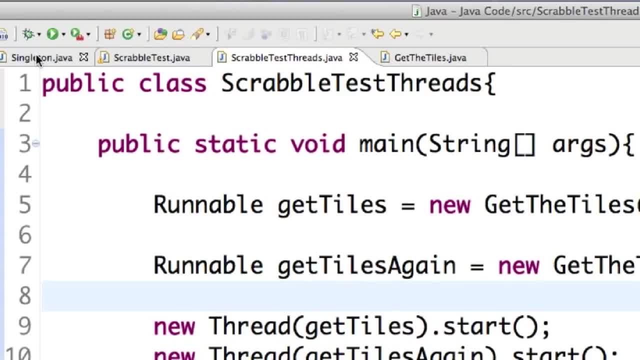 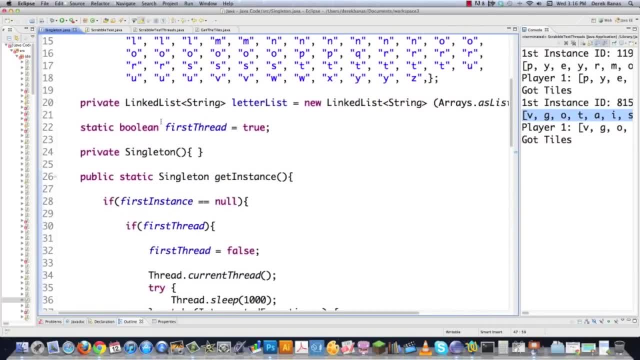 way. That's actually pretty easy, though, to come into singletonjava and fix all of that, which is exactly what we're going to do, So let's think about a couple different ways that we could fix that. So let's pull down inside of here and let's come to get instance. Now we very well could come. 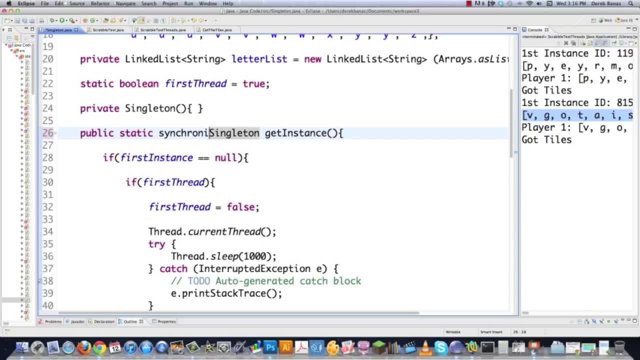 in here and change this to synchronized. Now, what this is basically going to do is it's going to force every thread to wait its turn. In essence, that way, only one thread is going to be able to access this method at a time, And until that thread releases this method being the get instance. 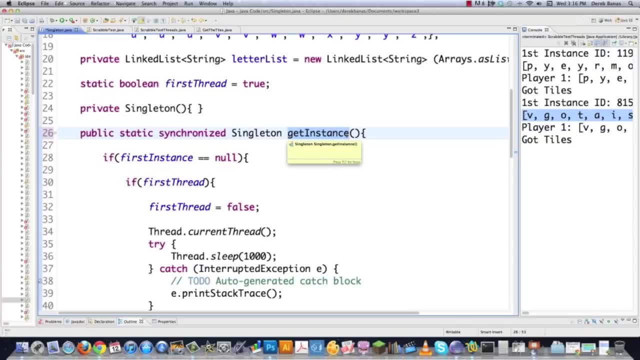 method which is going to create a new singleton object. no one else is going to be able to create a new singleton object. See, what happened here Was the first thread came in and it was told to go to sleep Meanwhile. since it's in here, 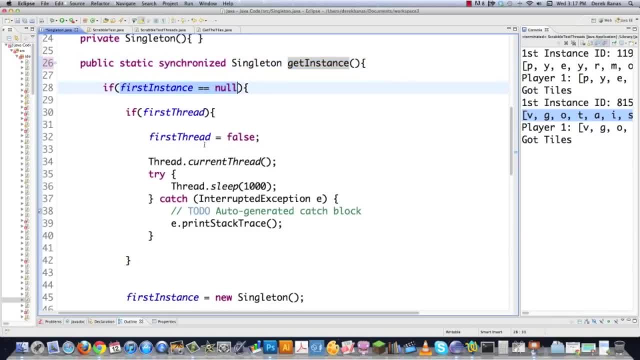 see this guy right here is checking to see if it's null. It went in here and then it fell asleep. Now, since it's set as null, that means there is no object that has been created from this singleton class, So we need to create a new one. Well, meanwhile, our first thread is right here. First, 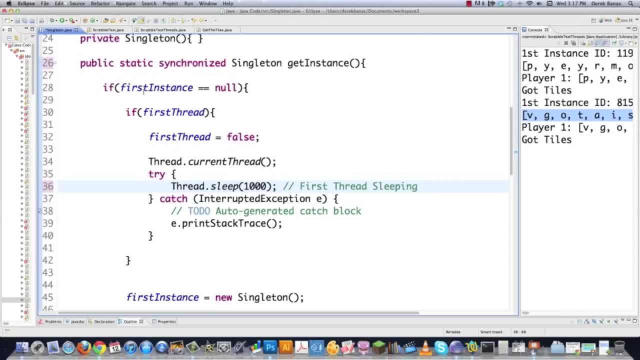 thread sleeping. So what happens whenever the second thread comes in and tries to create a new singleton object? it comes through right through the front door because, guess what, the first threads asleep down here and it goes in and creates another object, which is not what we 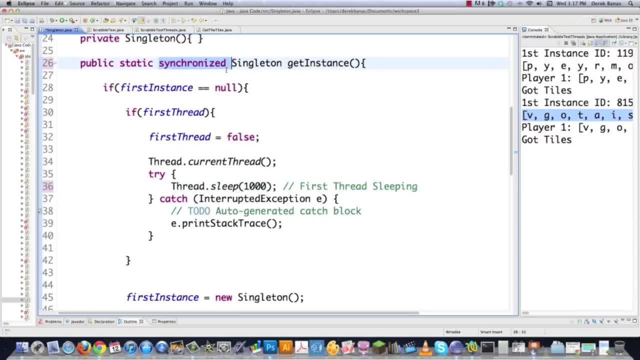 wanted to do. However, if we slap synchronized onto here, that is not going to allow this second thread to ever get in here until the first thread wakes up and then continues on to create the new object. However, we don't really want to use synchronized, because synchronized very often. 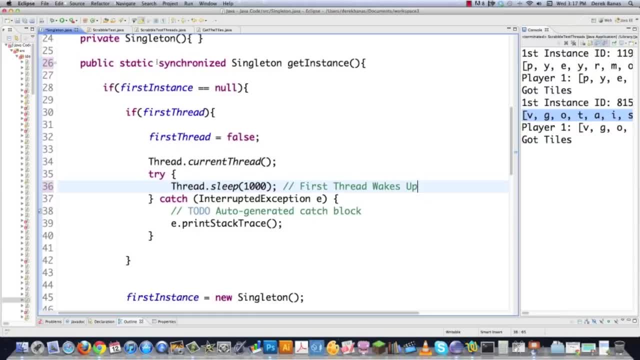 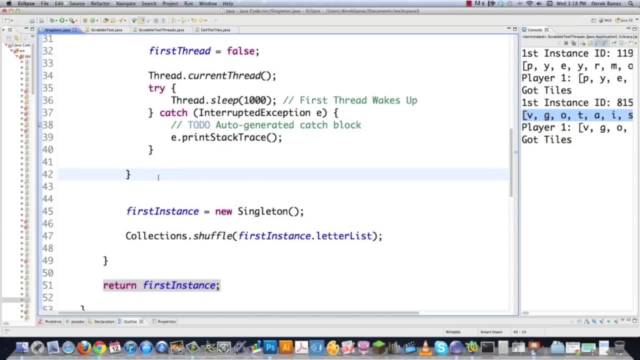 slows everything down dramatically. So in this situation, I'm going to show you another way to get the same results without slowing your program down, And it's actually going to be pretty simple. We're going to wrap everything inside of synchronized singleton class And, in essence, what this is going to do is this is going to force it to be a. 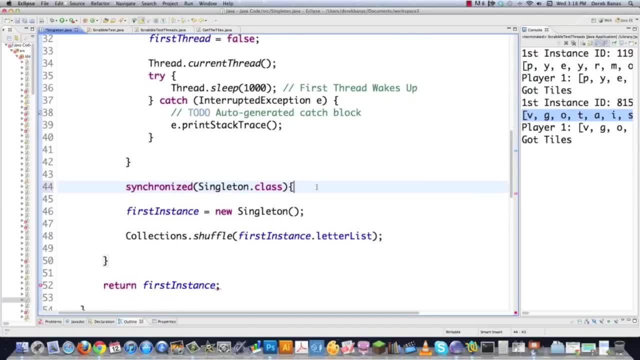 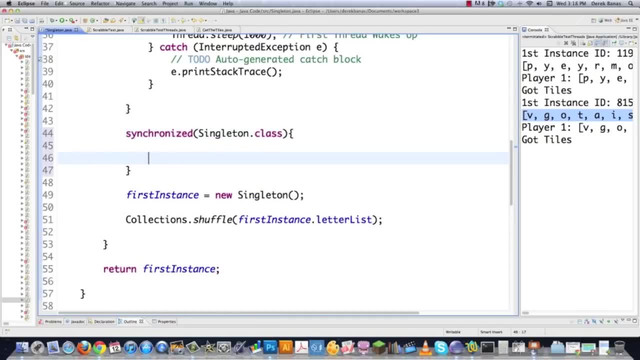 synchronized method until the first object is created, And then thereafter it is no longer going to be considered a synchronized class, And then, after this, we're going to run our same if statement. We're going to cut that out of there, paste it in there, and then we're going to check. 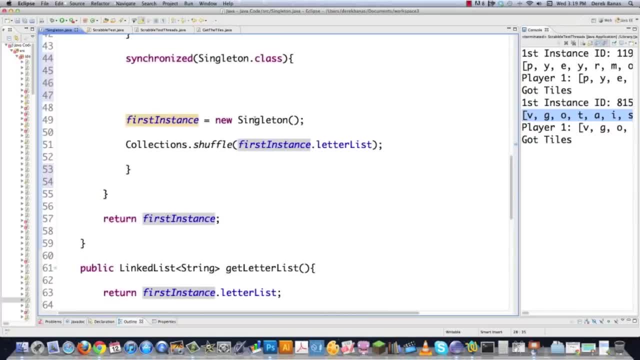 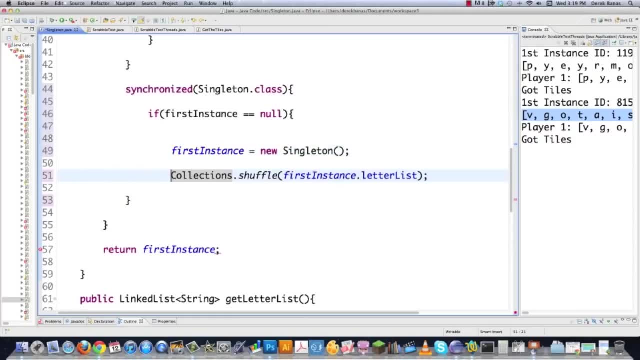 it for null again. Like I said, this is only ever going to happen. If we do that, we're going to have to wait for it to happen up until the very first object is created. And now we're going to go first instance and we're also going to shuffle our letters and then we're going to close off.